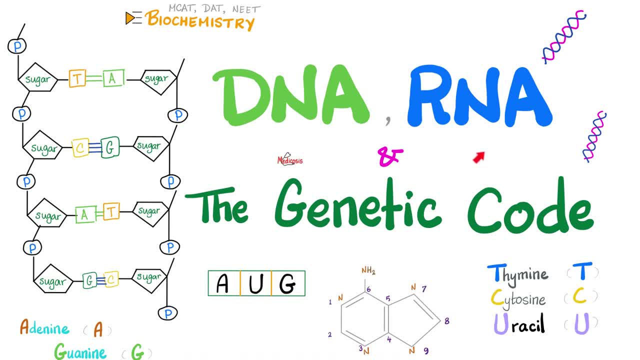 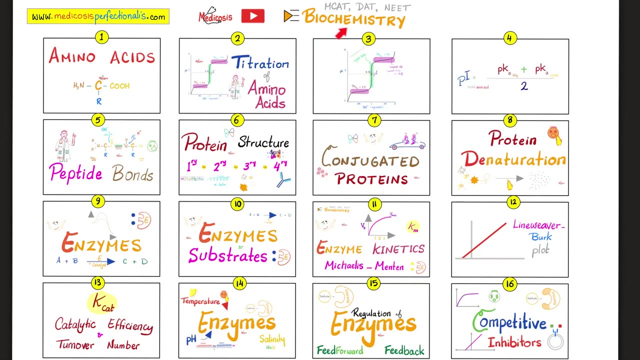 Today, let's leave the land of DNA and turn our attention to the land of RNA. Ribonucleic acid. What's the triad? The triad is the nucleotide, Ribosugar, nitrogenous bases and phosphate. Please watch the videos in this playlist in order. 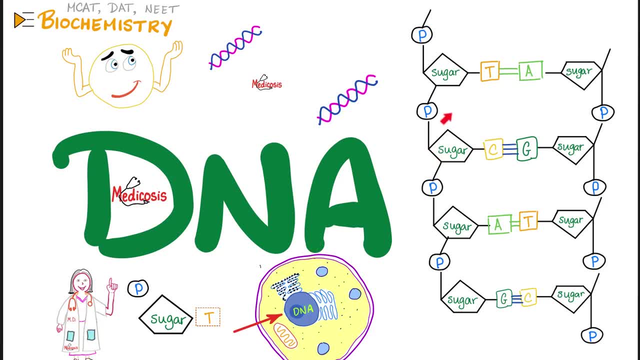 The DNA also had sugar base and phosphate, But the DNA has deoxyribosugar, whereas the RNA has just ribosucrate. There is another difference: DNA has thymine in it, but RNA does not have thymine Instead of 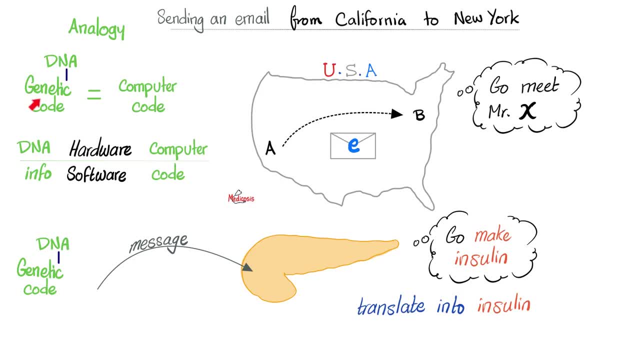 thymine RNA has uracil. Your genetic code is similar to the computer code. I want to send an email to a friend via a computer. The computer is the hardware, but the code is software. What's the hardware- Your DNA molecule- And what's the software? The answer is: it's the genetic code. 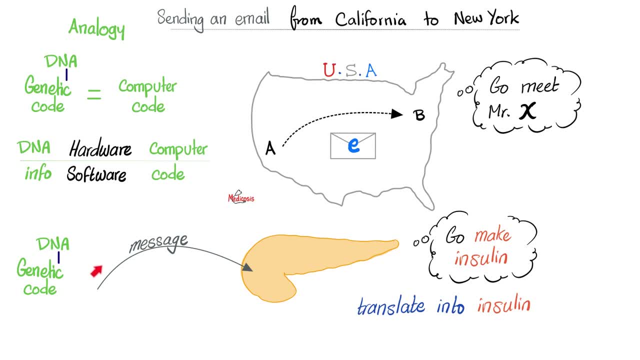 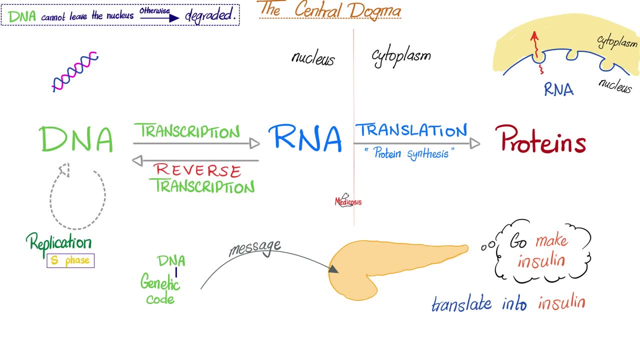 the organization of the DNA molecule Of the codons. Why are we trying to send a message? In order to make proteins. So that's the central dogma which we discussed before. When you double your DNA, it's called replication. When you convert DNA into RNA, it's called transcription. When you 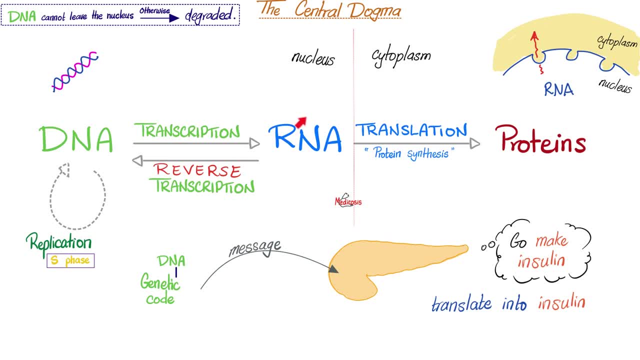 translate the message into meaningful proteins. this is called translation or protein synthesis. Your DNA is in the nucleus. It cannot leave. If it does leave the nucleus and go to the cytoplasm, it will be degraded in a second. If it does leave the nucleus and go to the cytoplasm, it will be. 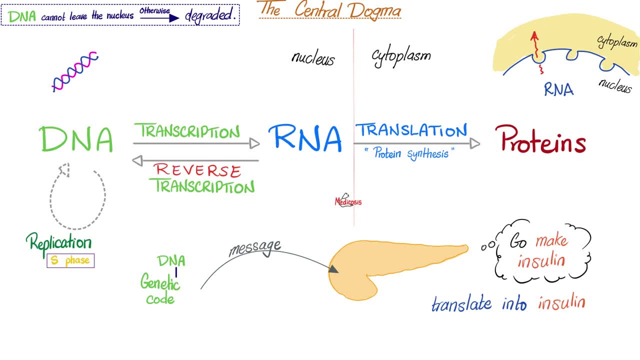 degraded in a second. If it does leave the nucleus and go to the cytoplasm, it will be degraded in a second. Who's going to take the message, then, from the nucleus to the ribosomes in the cytoplasm? Answer is RNA, especially mRNA. The messenger RNA is going to take the message from the nucleus to 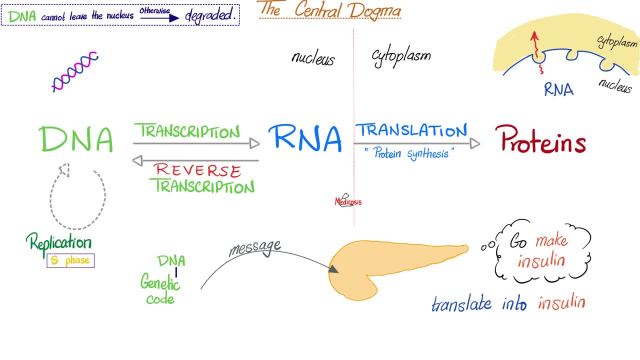 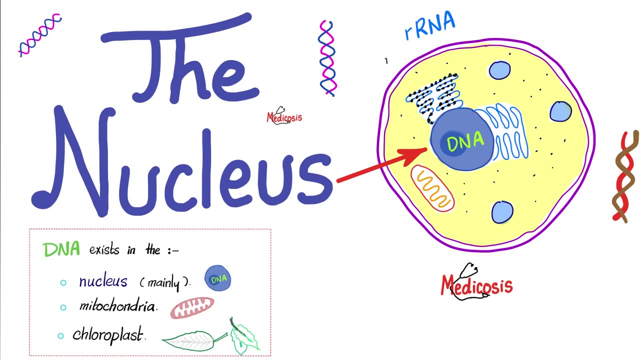 the cytoplasm by passing through the nuclear pores, My DNA is here in the nucleus And then the DNA copies itself called replication, And then the DNA will be transcribed into mRNA. The mRNA will take the message and will leave the nucleus via the nuclear pores until it goes. 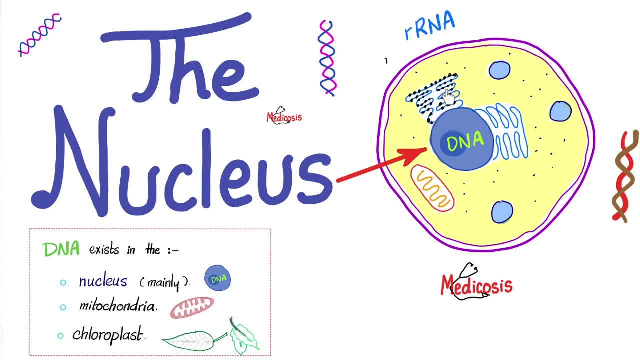 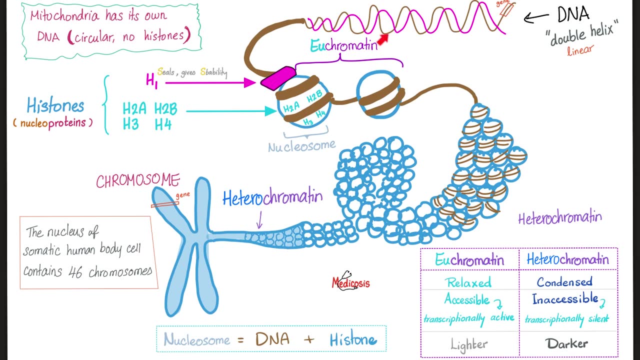 outside to find the ribosomes, usually on the surface of the rough endoplasmic reticulum- And then translation, which means protein synthesis, And that's how you code for proteins. In order for us to work on the DNA, the DNA has to be relaxed like this: in the euchromatin form DNA has. 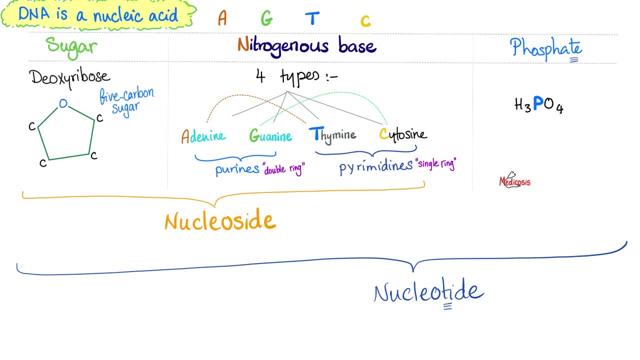 to be perfectly transparent and will apply觀眾 fibers to it, And there are tons of researchers who have influenced that. Here we have genetic studies that have shown that the response is totally different And, at the same time, the DNAарищes are anything apart from. 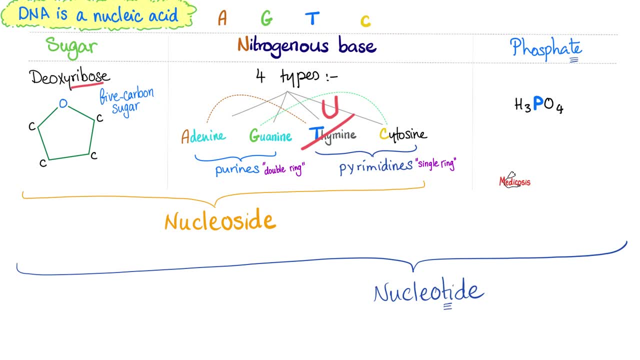 ulfHelp or double-diluty Uh, expand the regular growth pathway. We need to know that these things are totally uh at true level. Polylucatine PE- This is an freedoms that these compounds synthesizes DNA nucleotides- is called DNA polymerase, The name of the enzyme that synthesizes. 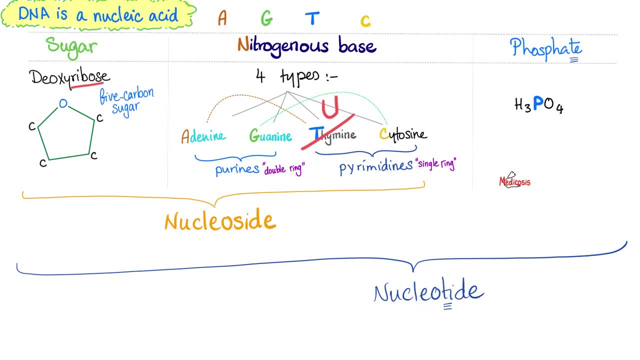 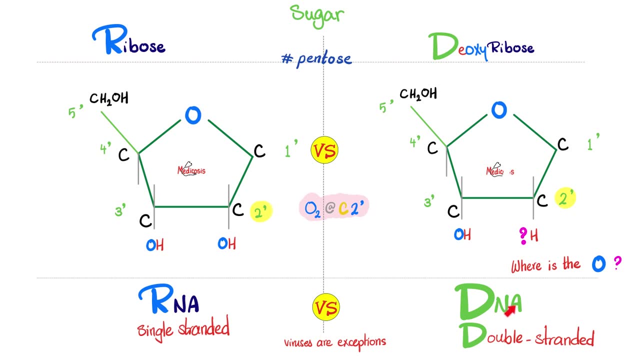 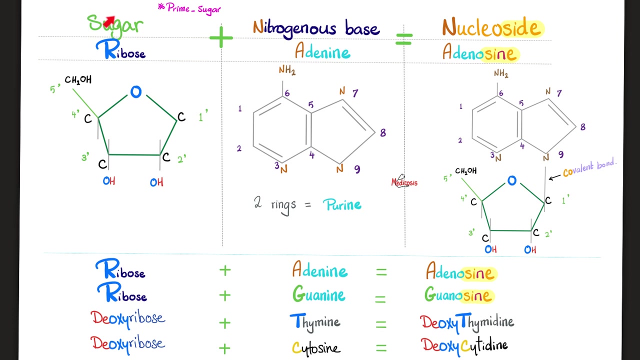 RNA. nucleotides is the RNA polymerase. DNA versus RNA. DNA has deoxyribose, RNA has ribose. DNA is double-stranded, RNA is single-stranded. Viruses are exception to this rule. Moreover, DNA has thiamine, but RNA has uracil. DNA cannot leave the nucleus, RNA can leave the nucleus Sugar plus. 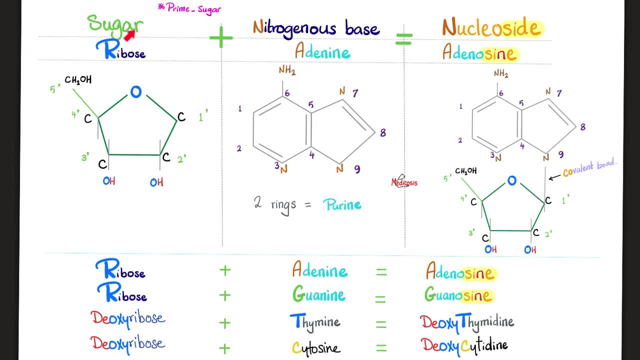 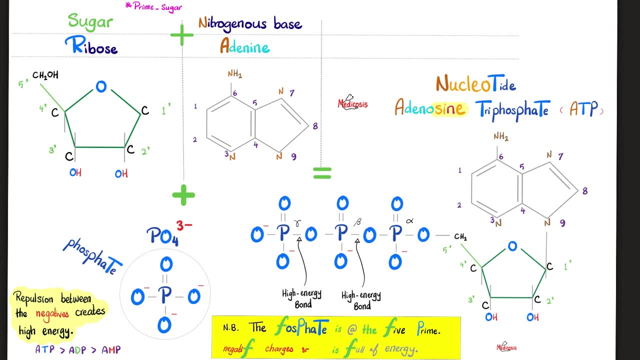 base equals nucleoside. Example: ribose sugar plus adenine, base equals adenosine, which is a nucleoside. Add a phosphate group to it, which is negatively charged, and before you know it, we have nucleotide such as adenosine triphosphate. Never, ever, forget that the phosphate is. 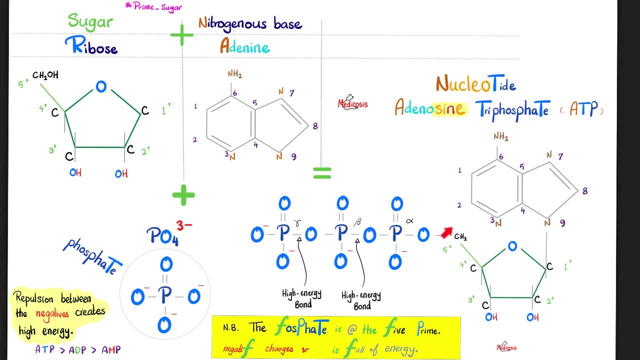 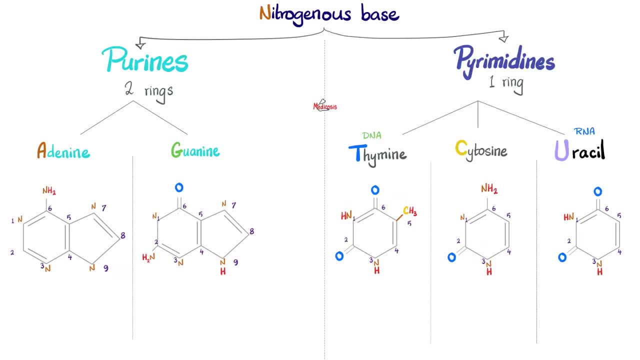 adenosine, The five prime, always the five prime. carbon Phosphate has a negative charge and phosphate is full of energy. These are the nitrogenous bases, pure as gold. The pyramid has one ring. Who are the pyramids? The rest of the shebang? Thiamine, cytosine, uracil. Thiamine is to DNA. what uracil? 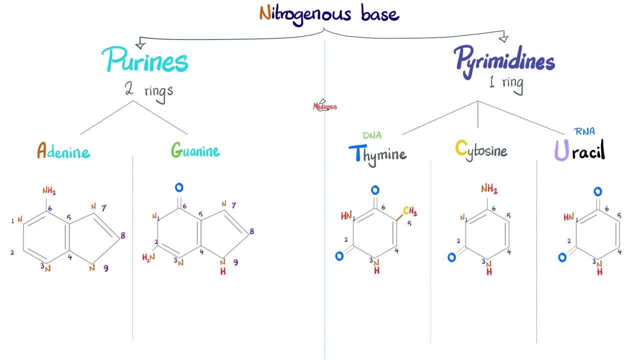 is to RNA. Please remember what we said before is that heat energy or thermal energy can convert the cytosine into uracil. Notice that cytosine has three nitrogen groups. Uracil only has two. Therefore, how do you go from cytosine to 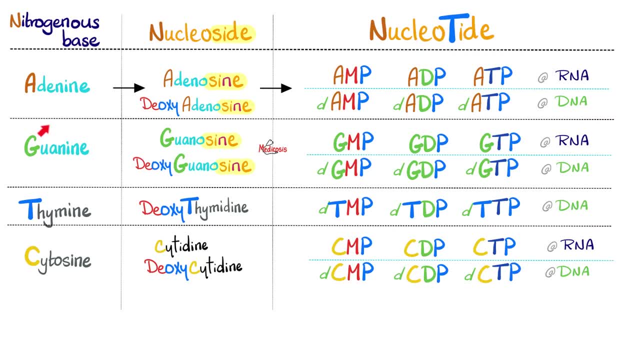 uracil. It's called deamination. Here is the base. Add sugar to it, It becomes nucleoside. Add one phosphate, You have monophosphate. Two phosphates: You have diphosphate. Three phosphates, You have. 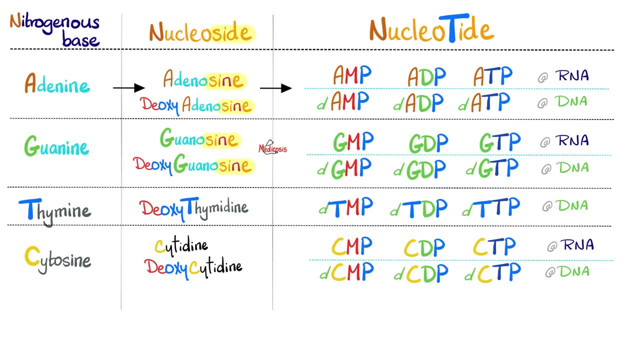 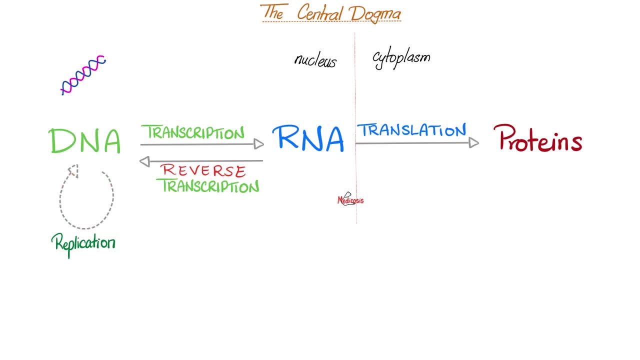 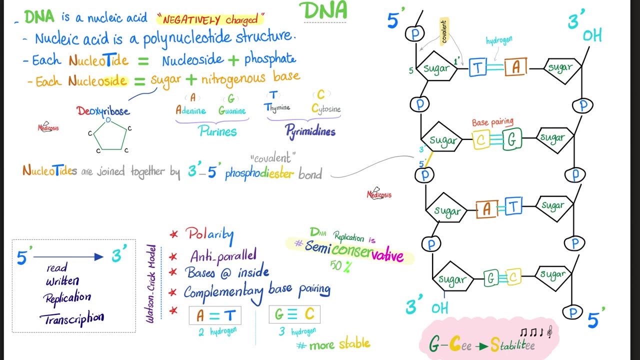 triphosphate. All of these are nucleotides. In a previous video we talked about DNA replication, which happens in the S phase of the cell cycle. Since phosphate at the five prime has a negative charge, your DNA as a whole is negatively charged. It's anti-parallel double helix, usually right-handed helix. The bases are: 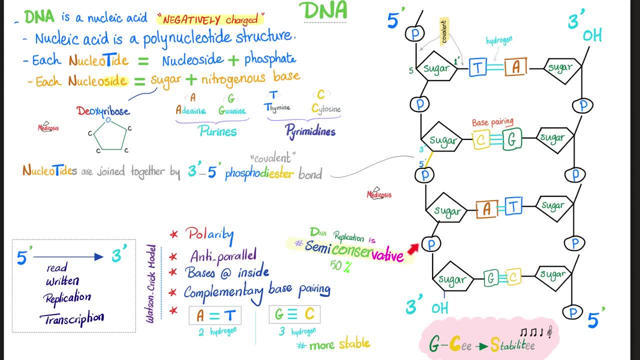 on the inside, but the sugar phosphate backbone is to the outside. RNA is similar, but instead of deoxyribose it's deoxyribose. So it's deoxyribose, So it's deoxyribose, So it's deoxyribose. 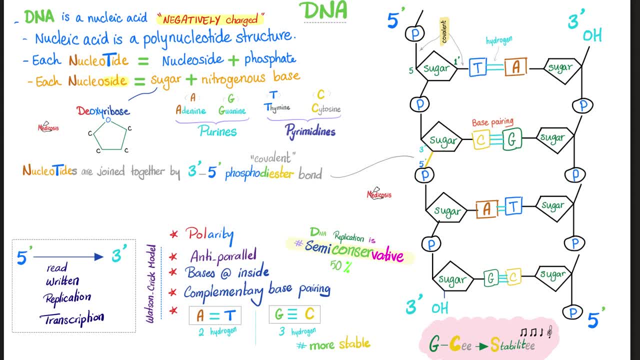 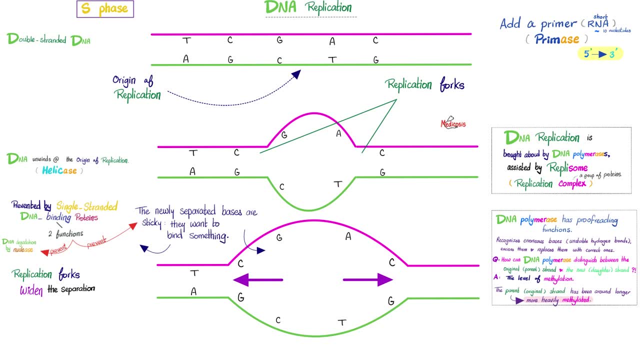 Instead of sugar we have ribose sugar, And instead of thymine we have uracil. And instead of double-stranded we have a single-stranded structure. DNA replication S- phase of the cell cycle. This is my original DNA. Each of these original parent strands will be copied to give. 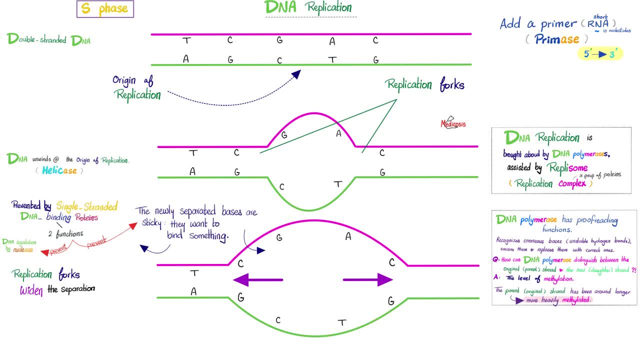 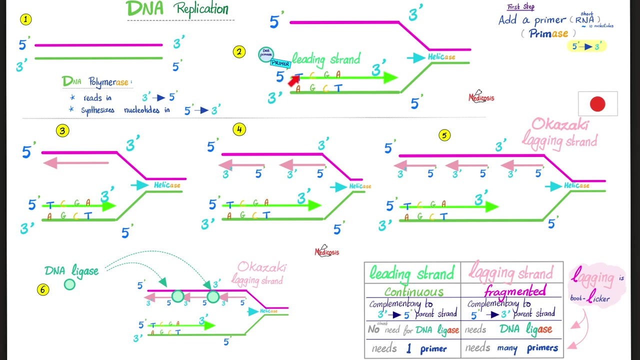 me two extra new daughter strands. We started the origin of replication, Open the replication fork. Fork back and forth in both directions. First step: the primase will add a primer, which is a short RNA molecule. DNA polymerase will add DNA nucleotides. The DNA polymerase synthesizes the new DNA from five prime to three prime. 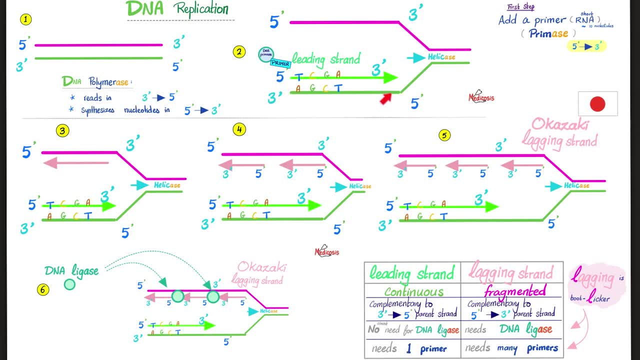 which means we have to read the three prime to five prime template In this direction. it will be one singular, continuous stride, known as the leading strand. But in the opposite direction we have the lagging strand with the single-stranded structure. So we have a single-stranded structure. 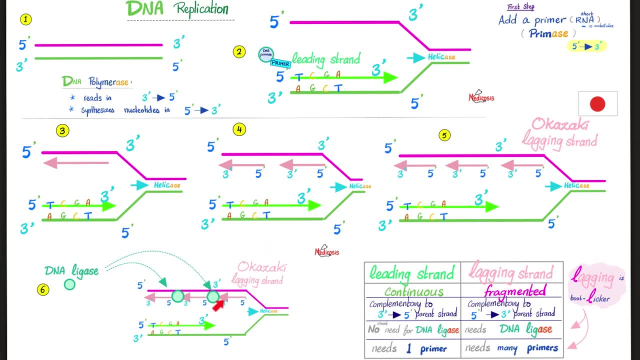 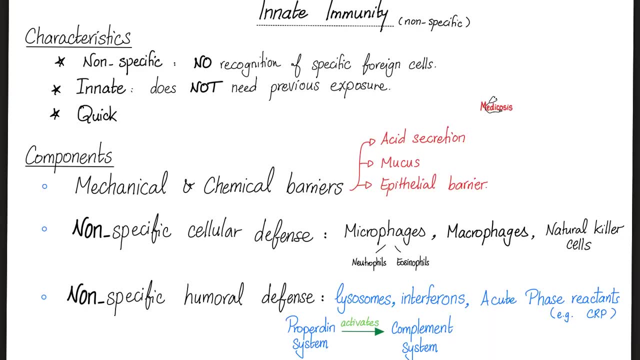 of the occasaki fragments which require DNA ligase to seal in the gaps later. This is DNA replication, which happens in the S phase of the cell cycle. Next, if you have watched my biology playlist, I've told you before about interferones. Why do we call them interferones? Because they 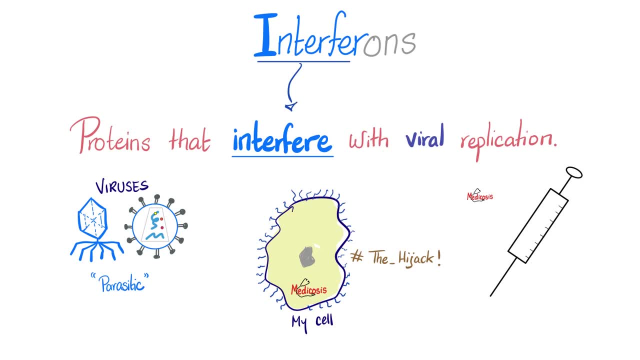 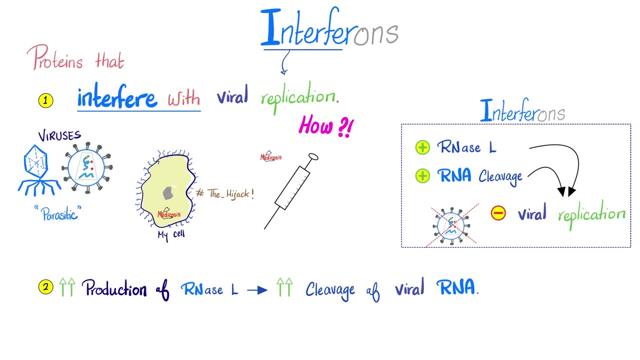 interfere with viral replication. What a beautiful name, But how did they do it? Well, they increase production of RNAs, which is an enzyme that breaks DNA. So if we have a DNA replication, we have to down rna so that the virus cannot replicate. remember: no rna equals no protein synthesis. 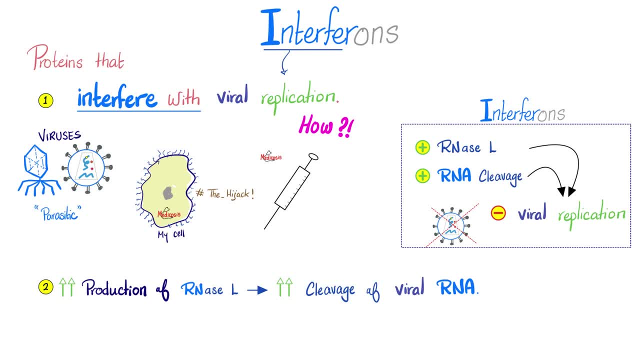 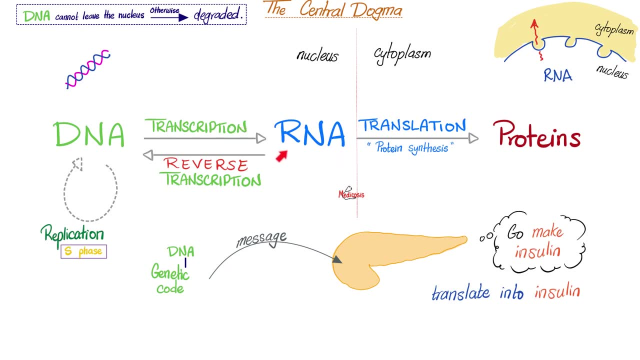 the virus without proteins is toast. go to hell. after copying that dna, let's use the copy that we just made. transcribe it to become mrna and then mrna will leave the nucleus through the nuclear pores. we'll go to the cytoplasm to find the ribosome translation will happen, which is 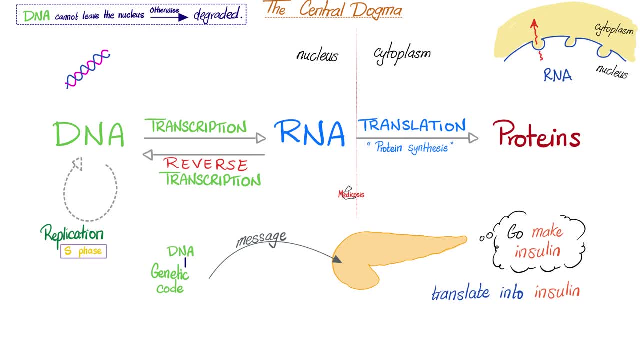 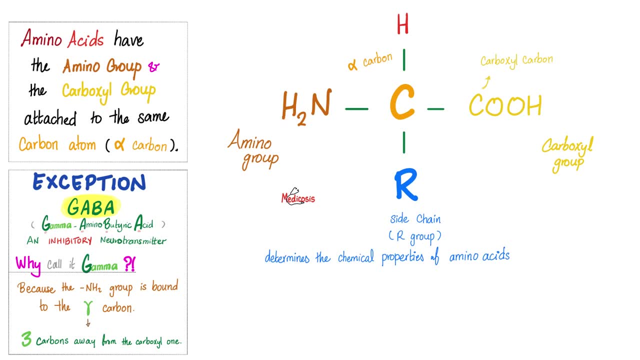 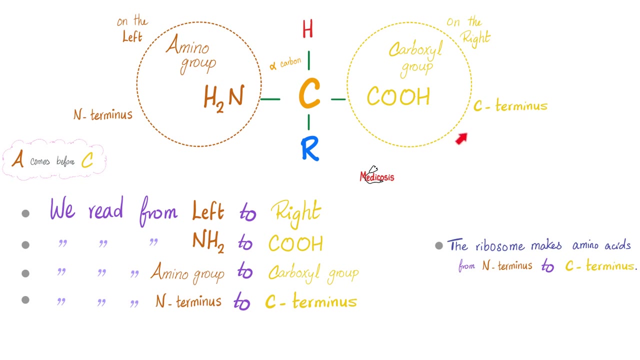 protein synthesis to make proteins. proteins are made of what? of amino acids, amino acid, amino carboxylic acid. that's why we call them amino acids. we read the amino acid from the left side to the right side, from the nh2 to the cooh, from the amino group to the carboxyl group, from the 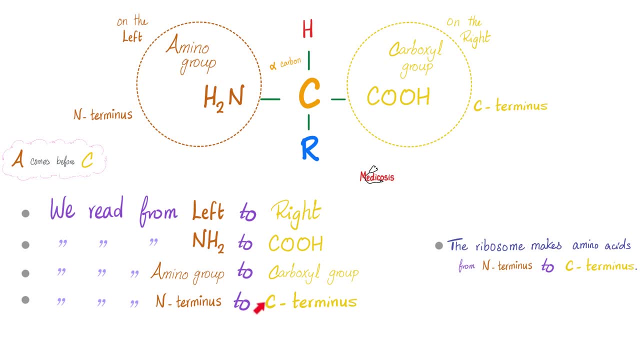 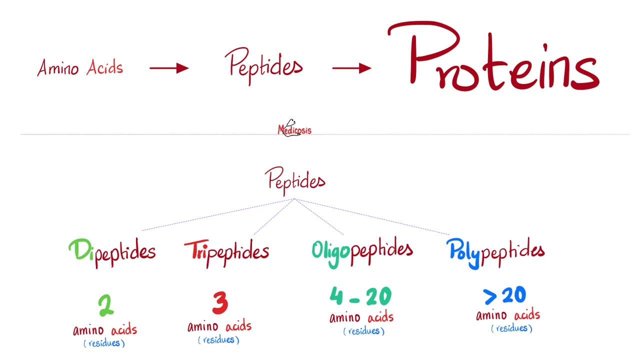 n-terminus to the c-terminus. why do we have to follow this rule? this some kind of a social construct? no, this is how your ribosomes make amino acids in real time. we put the n-terminus first, then the c-terminus. proteins are a bunch of peptides and peptides. 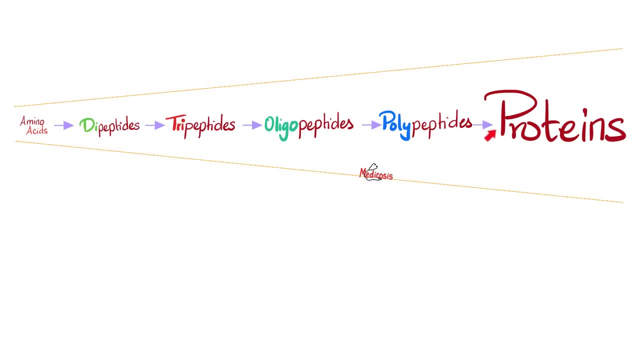 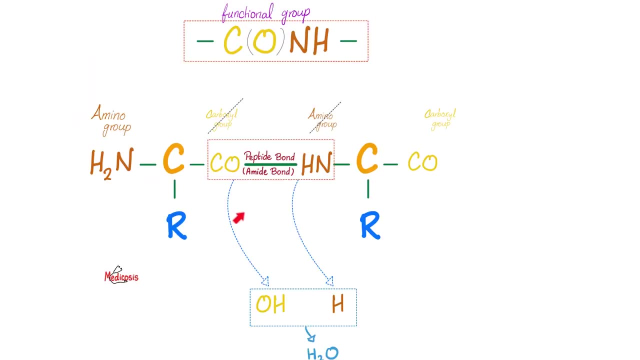 are a bunch of amino acids, so the building blocks of proteins are amino acids, and then you combine an amino acid with another amino acid. remove water, give me a lovely peptide bond, and now we have a dipeptide- repeat it again: tripeptide, oligopeptide, polypeptide, protein, etc. this is how. 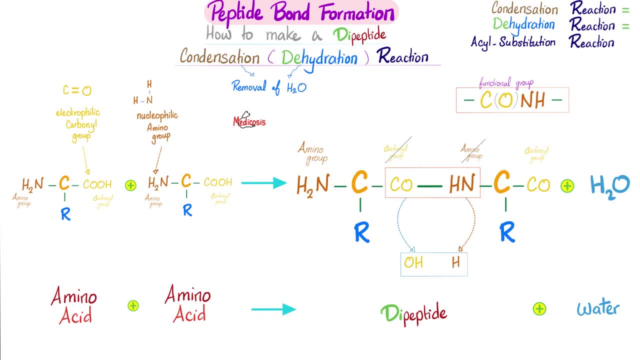 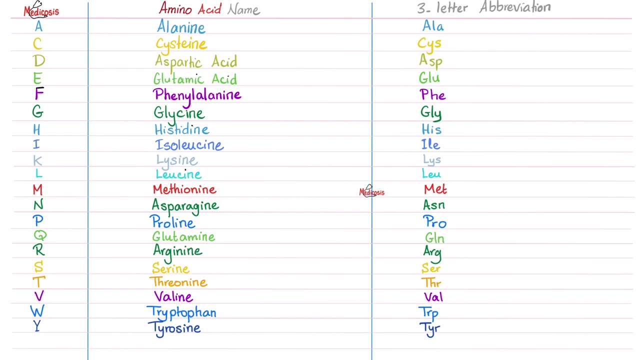 we make a peptide bond, releasing water in the process. it's a classic condensation reaction, because you're removing water. we've talked about this in previous biochemistry videos, so please pause and review how many amino acids exist in the universe? a lot, but how many amino 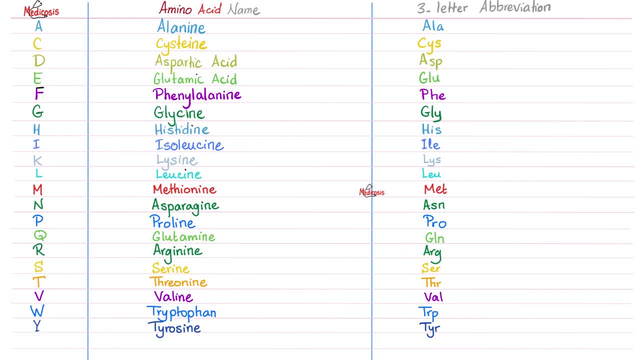 acids are coded for amino acids and how many amino acids are coded for amino acids. and how many amino acids are coded for by your genetic code? only 20.. each amino acid has a three-letter abbreviation and a one-letter abbreviation. you need to memorize the three-letter abbreviation at the very least. so turns out these: 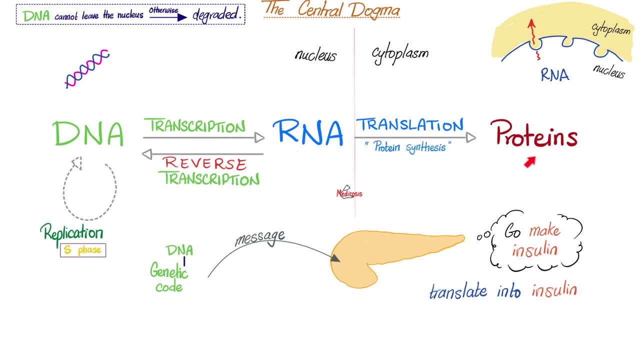 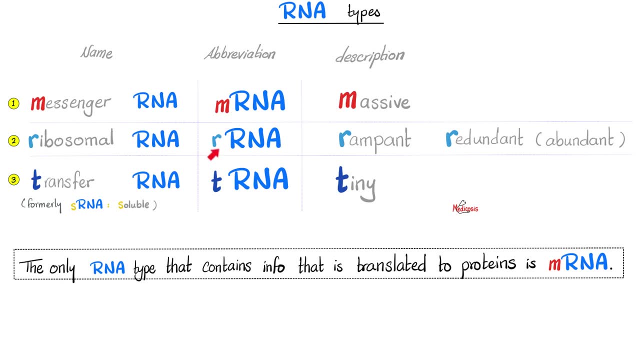 proteins are nothing but a bunch of amino acids linked together by peptide bonds, rna types. we have the messenger rna, we have the ribosomal rna and transfer rna, formerly known as srna, and transfer rna, which stands for soluble. which one is the biggest rna molecule? the m rna. it is 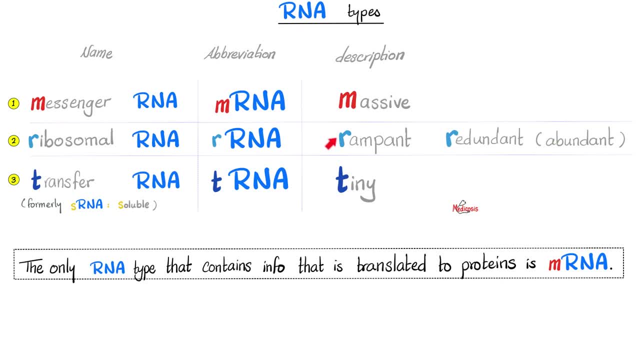 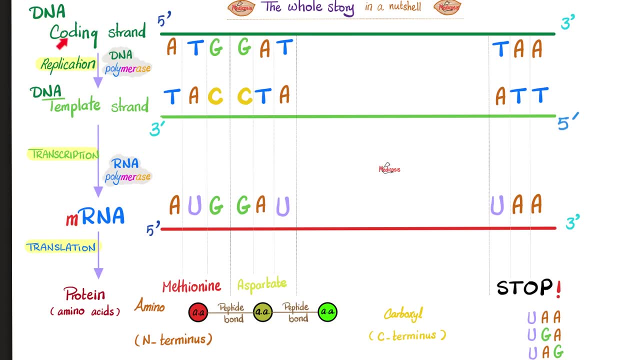 massive? which one is the most abundant or redundant or rampant ribosomal rna? which one is the tiniest molecule? t rna. this is my dna, right? yeah, start with one strand. call it the coding strand after replication. thank you so much. dna polymerase. we have another copy. let's call it a template. 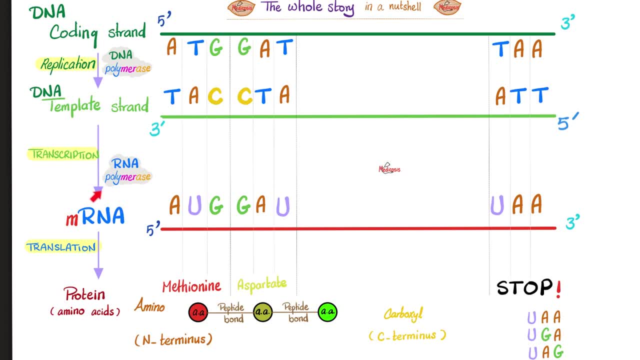 because this will be used as a template, to make a template, and then it will be used to make a RNA from it. How do you make RNA? How do you put new RNA nucleotides? By RNA polymerase, a polymer, many nucleotides together, The mRNA will leave the nucleus through the nuclear pores. It will go to 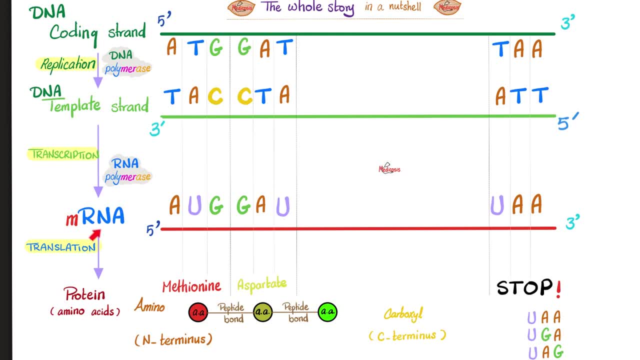 the outside, trying to find the ribosome, and then the ribosome will help us translate the message from meaningless codons into meaningful proteins. In order to build a house that has a specific shape and particular design, you need information first, and then we can materialize it as a house. 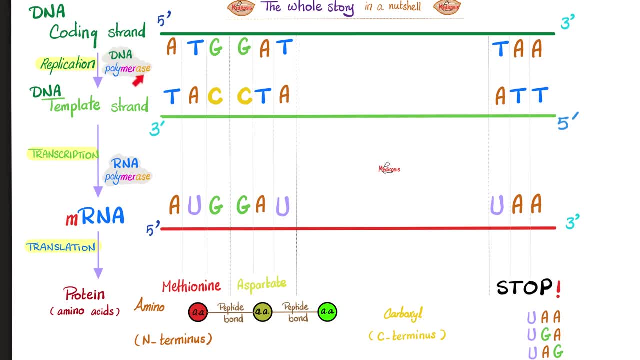 Remember that DNA polymerase synthesizes DNA nucleotides from the 5' to the 3' direction. Similarly, RNA polymerase will synthesize RNA nucleotides from the 5' to the 3' direction. But hey, Metacosis, why did you write 3' to 5' here? 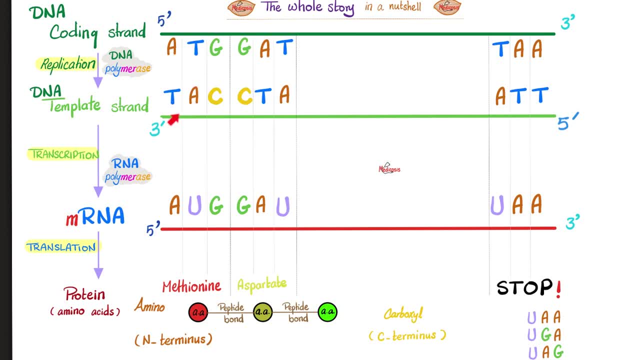 I had to write it this way so that it matches with everything above it and beneath it, But how it is made in real life is from 5' to 3' direction. Now let's play the game. Here is adenine on the DNA. The other strand is DNA. 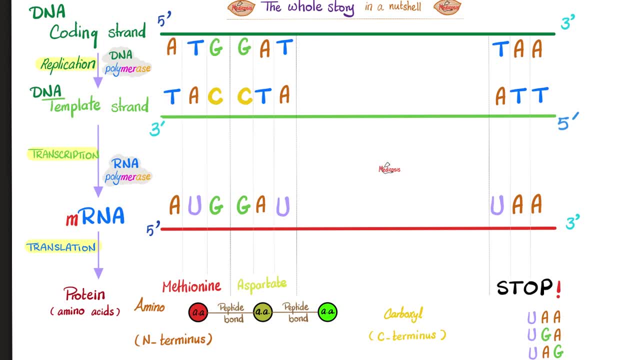 so A will be pairing with T, T with A, G with C, G with C, A with T, T with A. Then we'll take the template strand and try to make mRNA. The T should become A, A should become T, but there is no such thing as T on an RNA. Instead of T, say U. 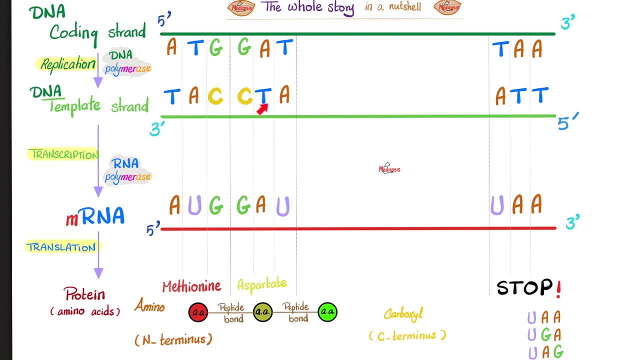 C becomes G. How about C, G, T, Right, fine, A, But A should become T. There is no such thing as T on an RNA. We'll say U instead Uracil instead of thymine Every time you see. 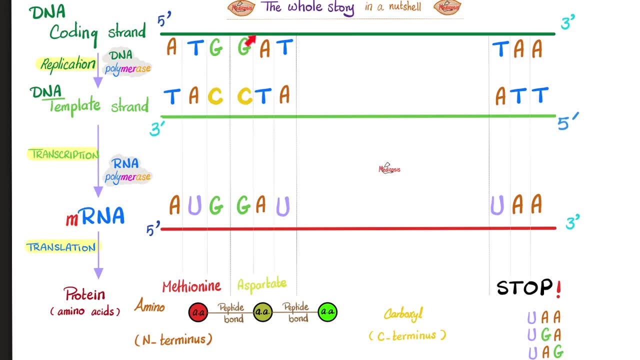 Uracil on the mRNA. it means it was thymine on the original coding strand of the DNA. But any time you see A on the mRNA it was an A on the original DNA strand. G was G, G was G But U was T. Next, look at this. Here is the codon. 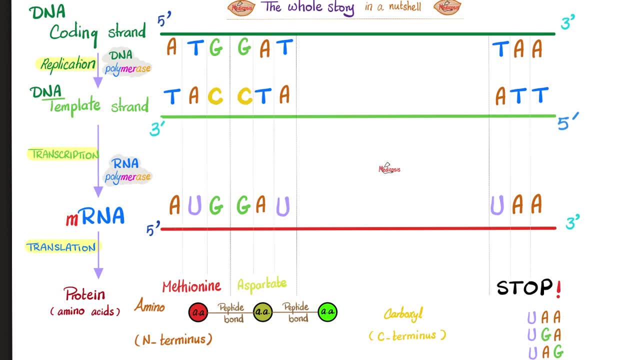 AUG. This sequence is important: AUG is not the same as AGU, is not the same as GAU, etc. The order is important, just like our daily language. This word is not the same as this word, even though they have the same letters, And then we'll translate the message: AUG. 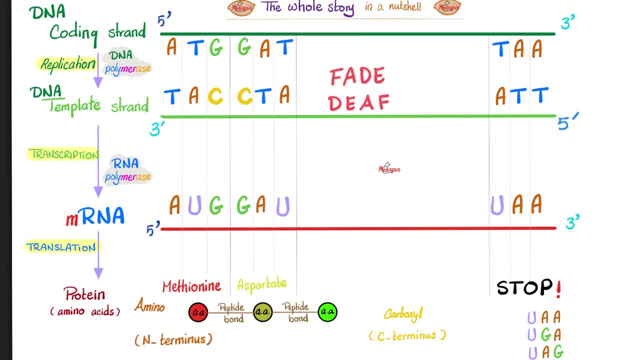 for example, will become the amino acid methionine, GAU will become aspartate or aspartic acid. And then you repeat it, you repeat it, you repeat it. Amino acid, amino acid, amino acid. Make a peptide bond. and now you're making a protein From 5' to 3' From the N'. 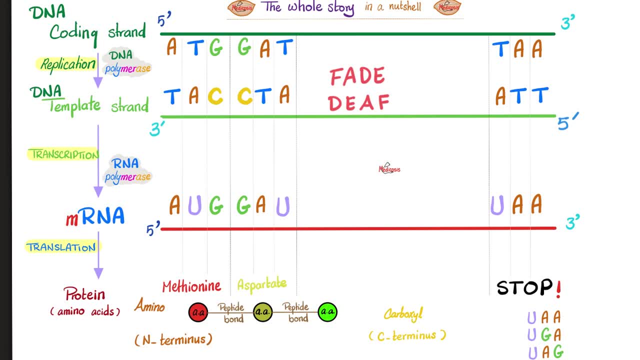 terminus to the C' terminus, Amino acid, And you will keep doing this until you hit one of these three stop codons. If you hit them, you will stop translation and the protein is truncated and terminated, and that's it. You need to memorize the first codon, AUG, which codes for: 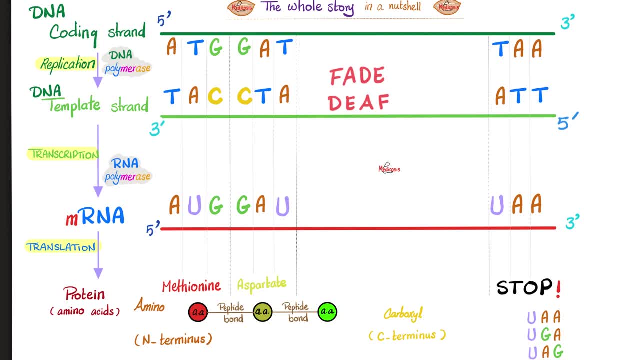 methionine, And you need to memorize the three stop codons, which are UAA, UGA and UAG. Please do not say UGG, because GG is a female's name and she is a hard-working person. She's. 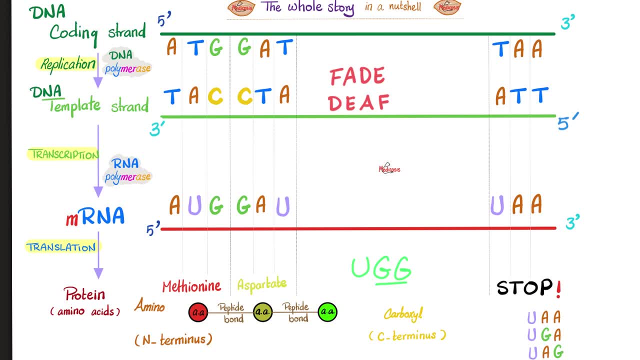 not gonna stop Mnemonic time. When the ribosome saw the stop codon, it said to the protein: you are away, You go away, You are gone, I'm done with it. But UGG is not a stop codon, You go. 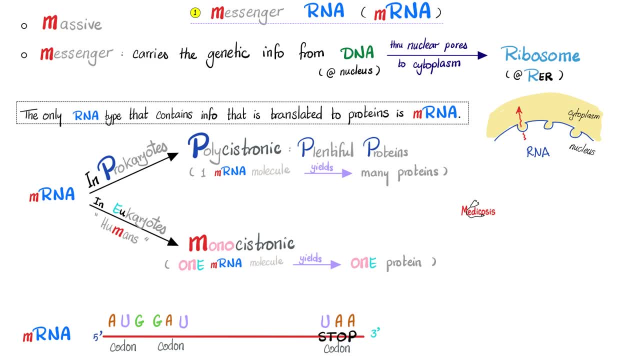 girl. Let's talk about each type of RNA briefly, And then in the next video we'll dig deeper. mRNA is massive. It's the messenger. It carries the code, the message from the DNA which is in the nucleus, And then we'll go to the ribosome. 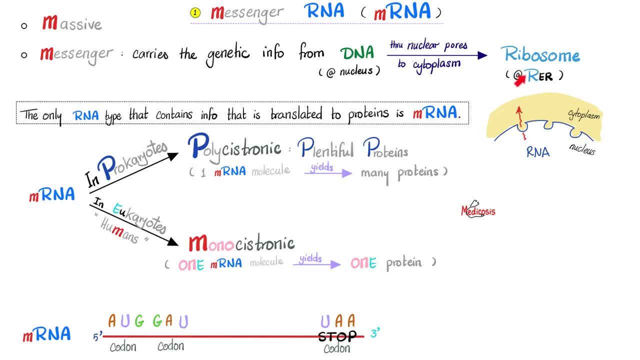 which is outside the nucleus, Could be in the cytoplasm or on top of the rough endoplasmic reticulum. That's why the rough endoplasmic reticulum is rough because of the ribosomes, The only type of RNA that contains genetic info of that is translatable to proteins. 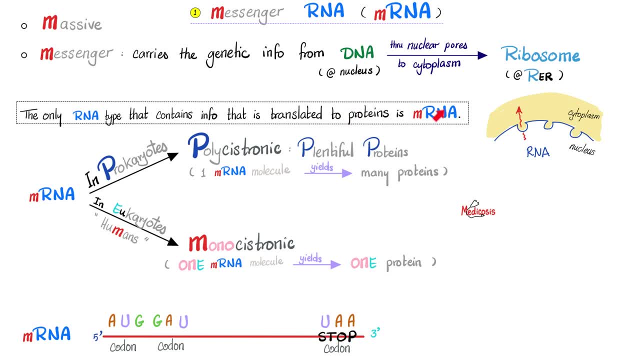 is mRNA. rRNA cannot do it, tRNA cannot do it. mRNA in prokaryotes is polycistronic. What the flip is that Poly means many, Cis means the same. The same Singular mRNA molecule is giving me. 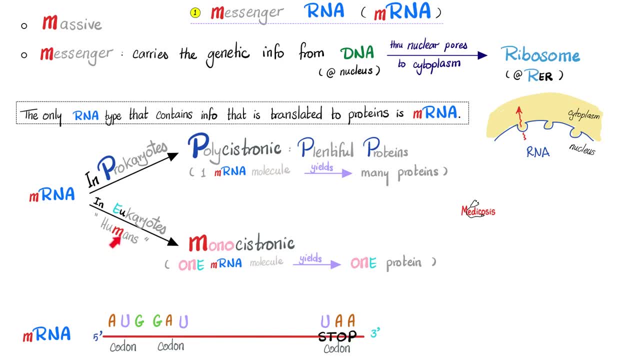 tons of proteins, Poly, But in humans, you and me- we are eukaryotes, And in eukaryotes mRNA is monocystronic. One mRNA molecule can only give you one protein. In the real world, mRNA한다 is just a simple purple protein, Not any other protein. 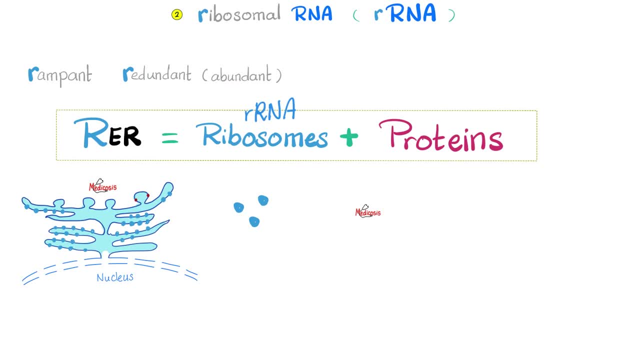 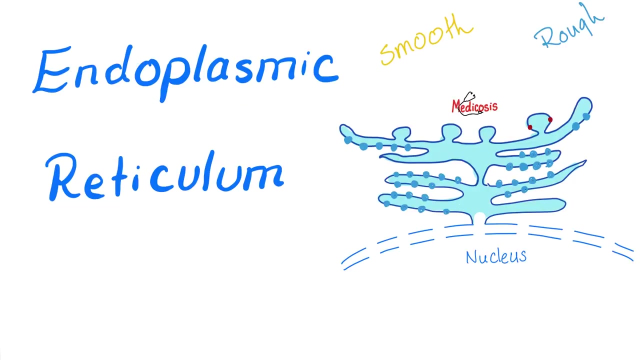 Next, ribosomal RNA, The most abundant RNA type. Never, ever, forget this. the rough endoplasmic reticulum equals the ribosomes plus proteins. What does the ribosome have? Ribosomal RNA. If you want to learn more about the endoplasmic reticulum, check out the video titled. 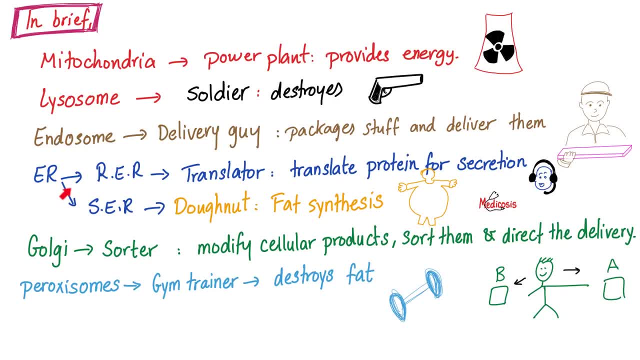 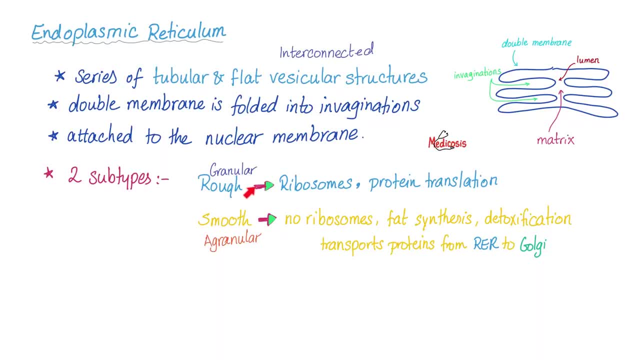 Endoplasmic Reticulum. in my biology playlist, Endoplasmic Reticulumricht43 could be or smooth. Rough is for translation, which means protein synthesis. Why is the rough rough? Because it's ribosomes. The ribosomes is giving it its granular shape. Function of the rough endoplasmic. 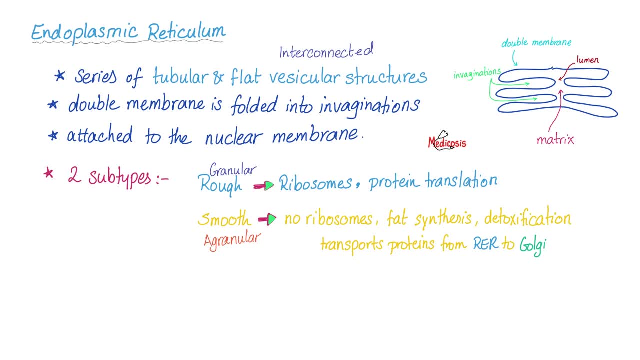 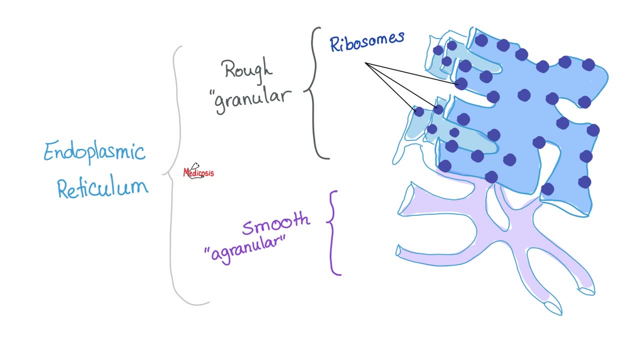 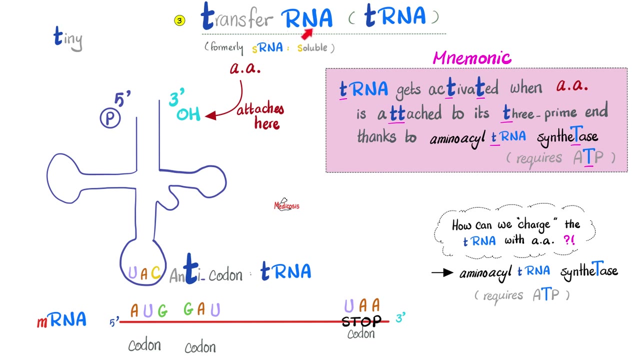 reticulum is protein synthesis or translation of mRNA into proteins. This is the rough endoplasmic reticulum, which has ribosomes which have rRNA. and this is the smooth endoplasmic reticulum: no ribosomes and no rRNA. The third type transfer RNA or tRNA. It looks like a clover. 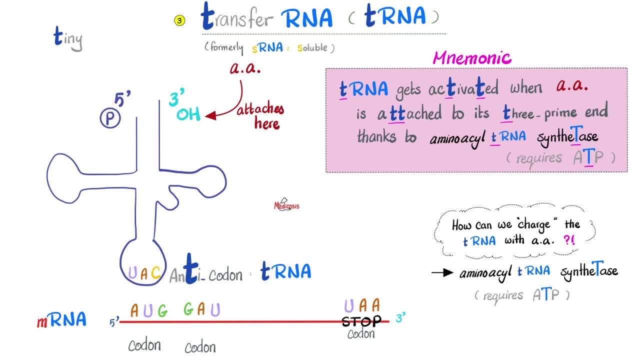 leaf. It has a 5' with phosphate again and 3' with OH. Where will the amino acid fit? The amino acid will fit into the 3' end And the part of the tRNA that will meet with the mRNA and pair. 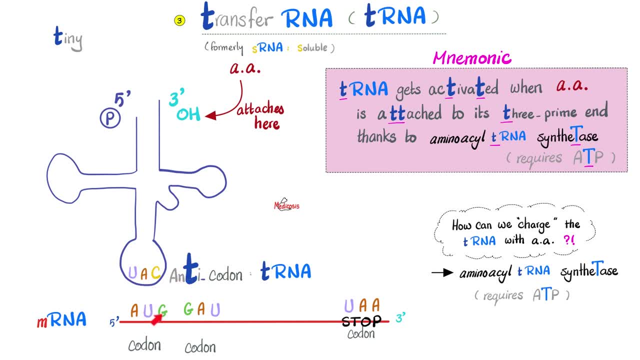 together is called the anticodon. which pairs with the tRNA And the tRNA that will meet with the tRNA and pair together is called the anticodon. which pairs with the tRNA And the tRNA that will meet with the tRNA and pair together is called the.